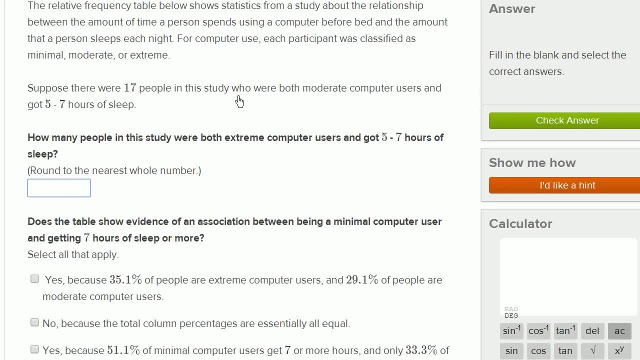 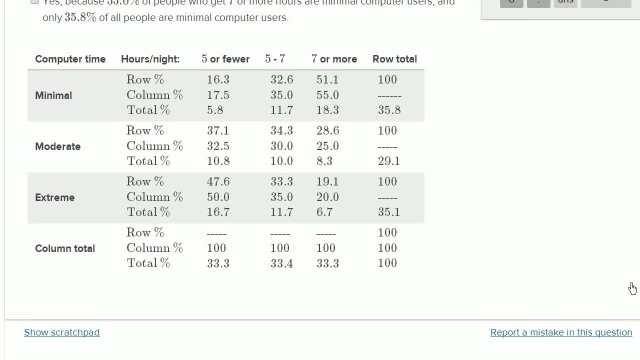 So they tell us suppose there were 17 people in the study who were both in moderate computer users and got five to seven hours of sleep. So moderate, five to seven. So this category right over here. there were 17 people in this category over here. 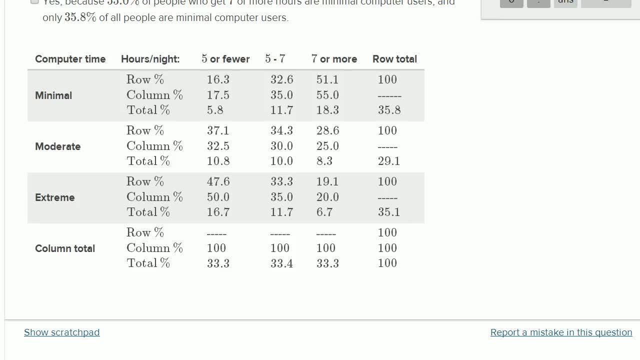 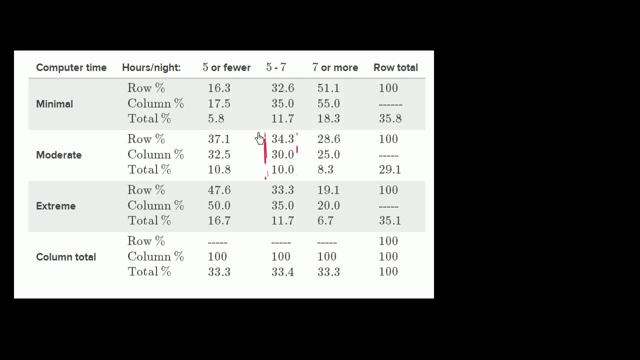 And just to mark that, let me, I copied and pasted this chart. I copied and pasted this chart onto my scratch pad so I can write on it. So this group, they're telling us this group, and my pen is really acting up. 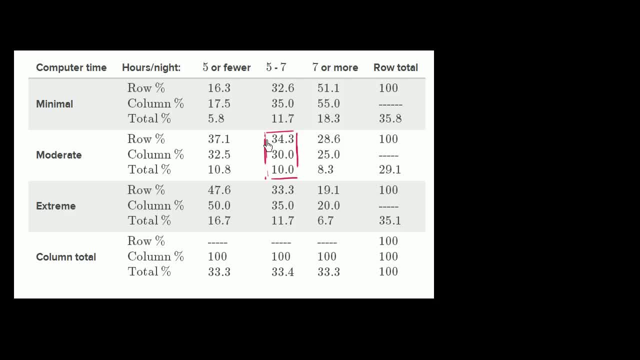 I don't understand what's going on. This group right over here, there are 17 people. So that group right over there is 17 people. Now what are they asking us? They're saying so. they're saying how many people in the study? 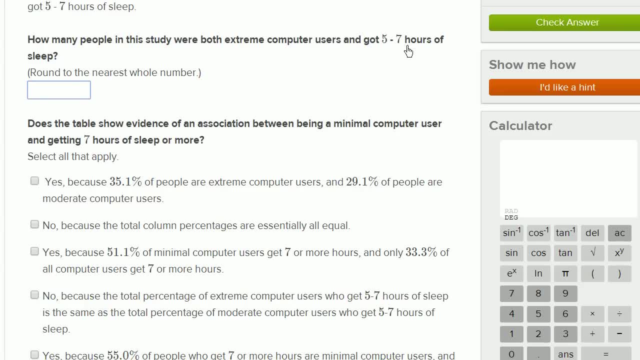 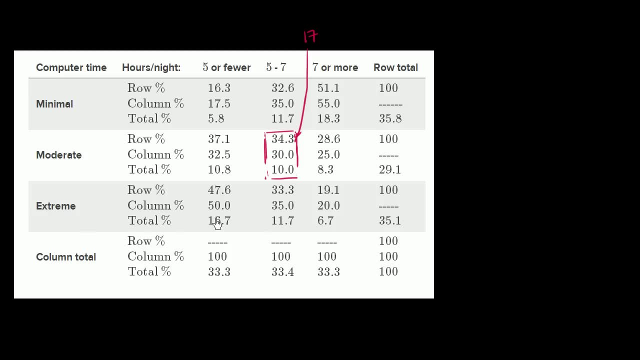 were both extreme computer users and got five to seven hours of sleep around to the nearest sleep. This whole number So extreme and got five to seven. Get my scratch pad out. So they're saying how many people are in, how many people are in this bucket. 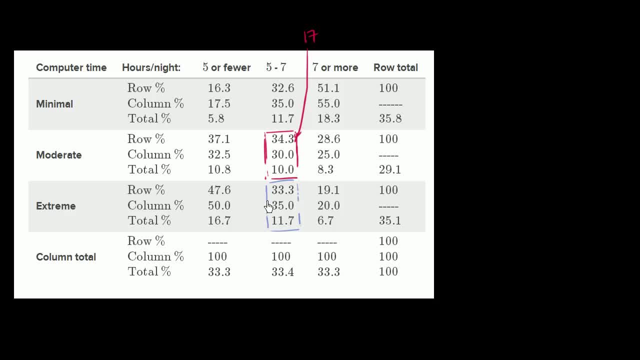 in this bucket right over here. I think I have to replace my pen tablet or something. I don't know why it's getting all splotchy like this. So how would we think about this? There's 17 people in this group. 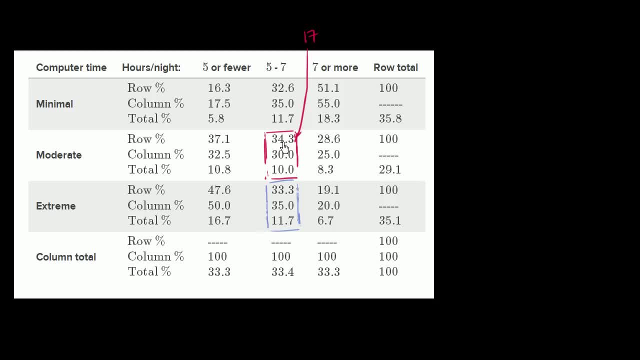 How many people are in this group? Well, they tell us that 17 is 34% of the row total. so I guess you could say 17 is 34.3% of the moderate, of the moderate computer users. Or you could say that 17 is 30% of the people. 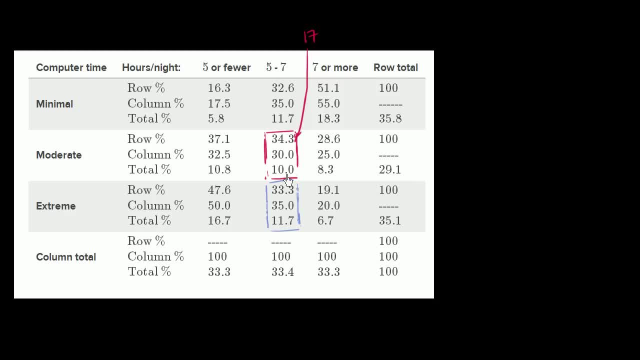 who slept five to seven hours each night. Or you could say 17 is 10% is 10% of the total of the total number of people. So let's just go with that. We could figure out the total number of people. 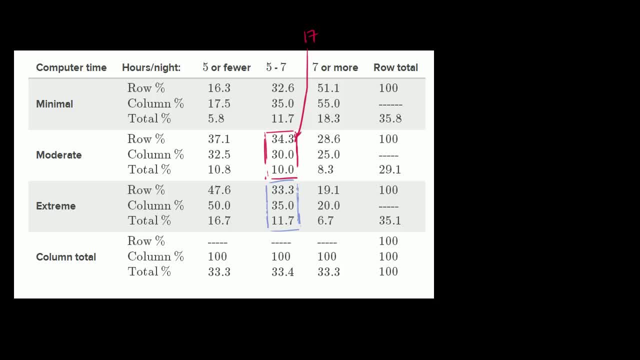 So 10%, actually. let me write it this way: So 10%, 10% of the total, 10% of total is going to be equal to 17,. or that the total just divide both sides by 10% is equal to 17. 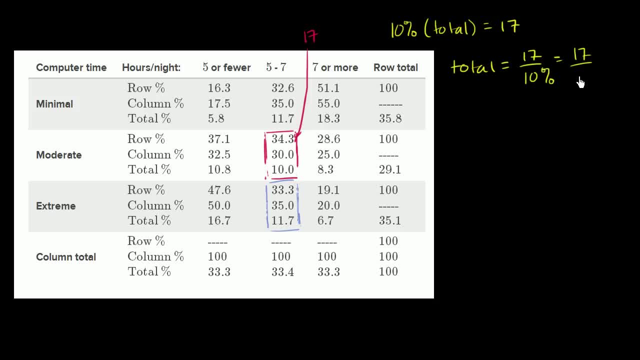 divided by 10%, which is the same thing as 17 over 0.1, which of course is equal to 170.. So the total is 170, and they tell us that extreme, extreme computer users represent extreme computer users who sleep five to seven. hours per night represent 11.7%, 11.7% of the total. So to the answer to their question of how many people were extreme computer users who sleep five to seven hours per night, it's 11.7% of 170.. 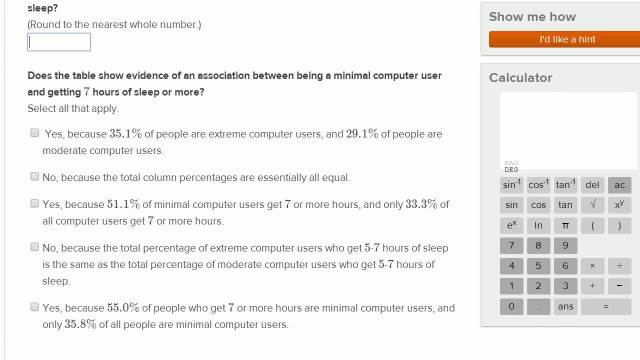 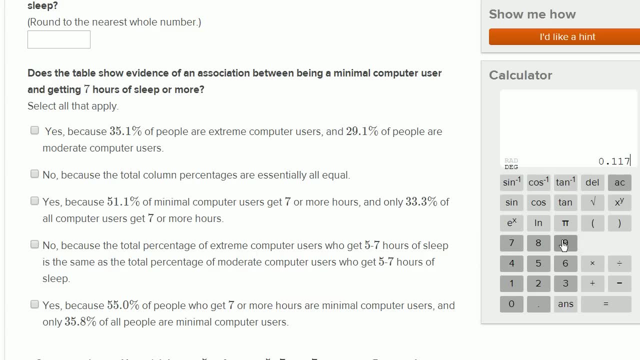 So let's go back over here So we actually have a little calculator tool here. So it's 11.7%, which is 0.117, times 170.. And let me make sure that you can see what I'm doing by scrolling over a little bit. 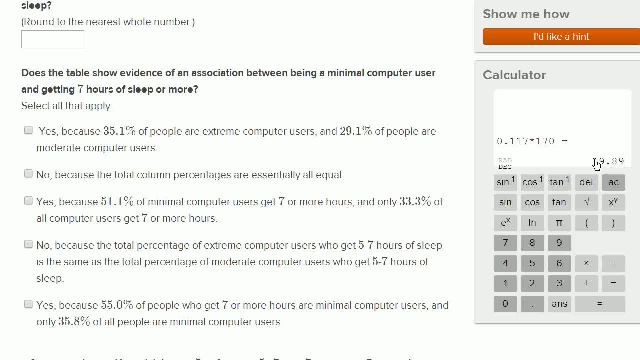 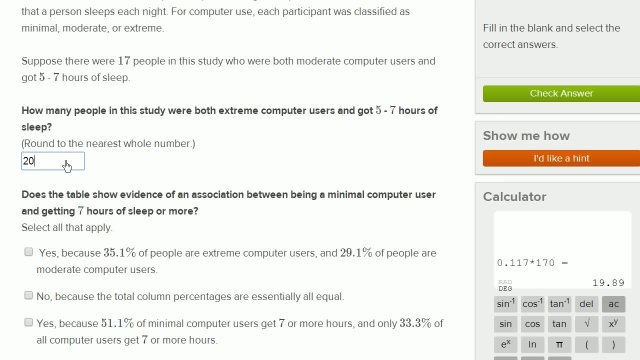 Times 170 is equal to 19.89.. So if we're rounding to the nearest whole, that's going to be 20 people. And then they are going to ask us some questions. They say: does the table show evidence? Does the table show evidence of an association? 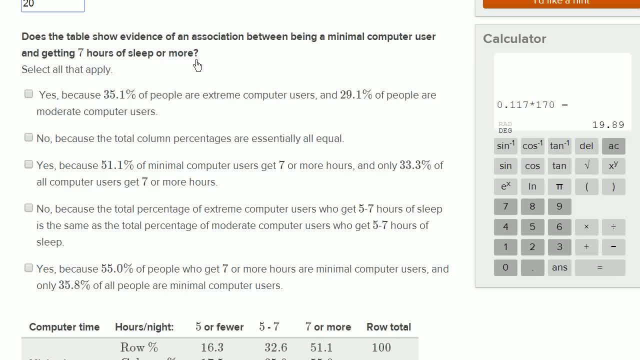 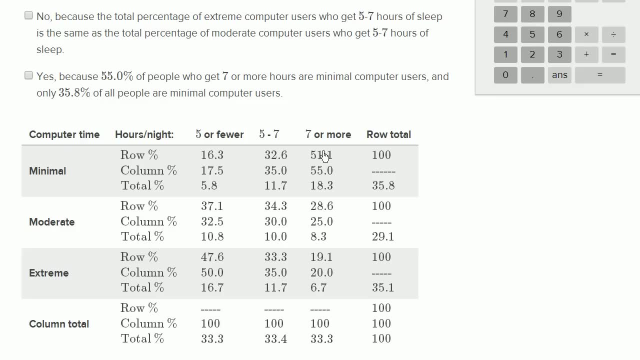 between being a minimal computer user and getting seven hours of sleep or more. So let's just look at the chart. So an association between being a minimal computer user and getting seven hours of sleep or more. So it looks like minimal computer users. so these are the minimal computer users who get. 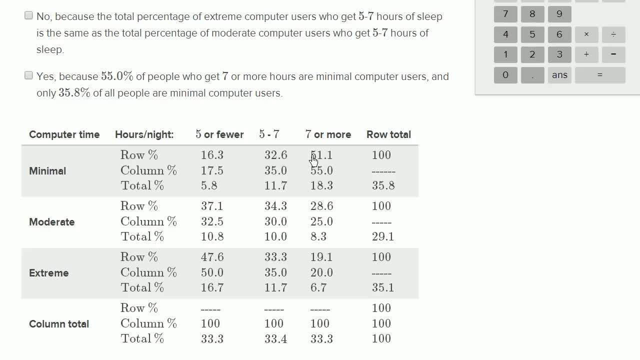 seven or more hours of sleep, And there's a couple of ways to read this. So you could say that 51% of minimal computer users get seven or more hours of sleep. You could say that of the people who get seven or more hours of sleep, 55% are minimal computer users. 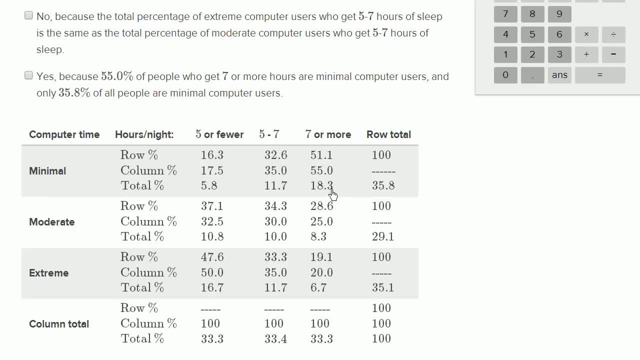 And of course, this one just says that minimal computer users who get seven or more hours of sleep represent 18.3% of all of the people who were surveyed. So let's look at the choices. And when I just actually, before I even look at the choices. 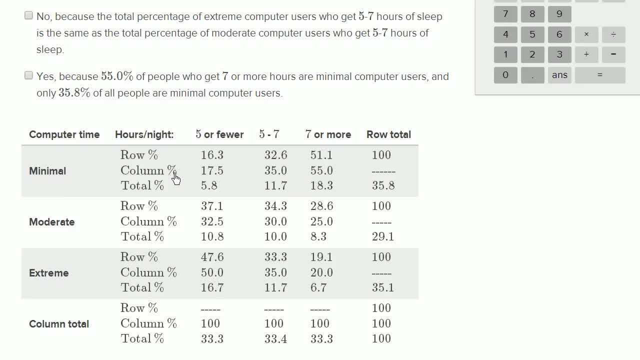 let's see if there's an association. It does look like. if you look at minimal computer users, it looks like a small percentage. only 16% get five or few hours, A higher percentage gets five to seven hours And 51%- the highest percentage gets seven or more. 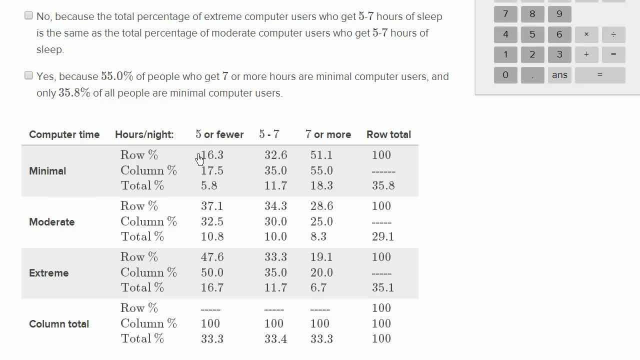 So it looks like for minimal computer users. it looks like the distribution is definitely weighted towards getting more sleep And, for example, if we look at the extreme computer users, it's the opposite trend: 47% have five or few hours per night, 33% five to seven hours. 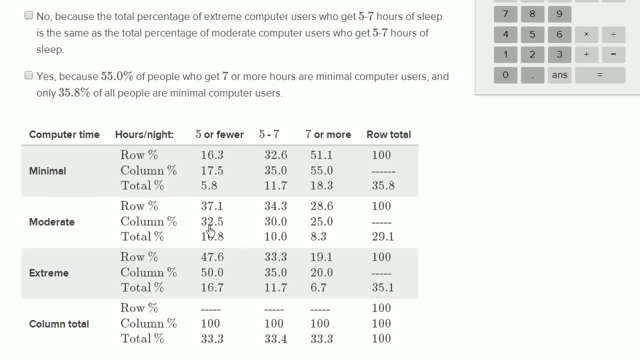 And then only 19% get seven or more, And it looks like the moderate is someplace in between. So just looking at this, just looking at each of these rows, it looks like there's a trend where, if you use a computer for less time, 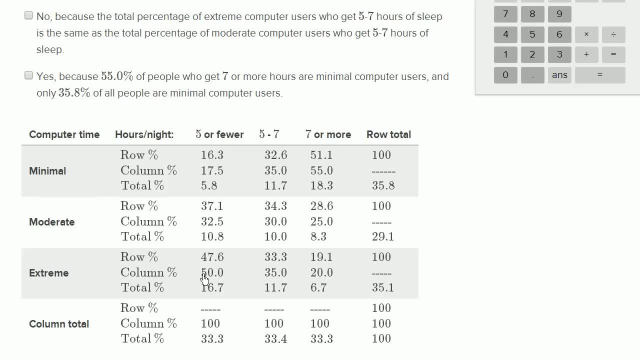 you're more likely to have more sleep, And likewise, if you use a computer more, you're more likely to have less sleep. Another way to think about it: when you look at the people who are getting seven or more hours of sleep, a majority of them are minimal computer users. 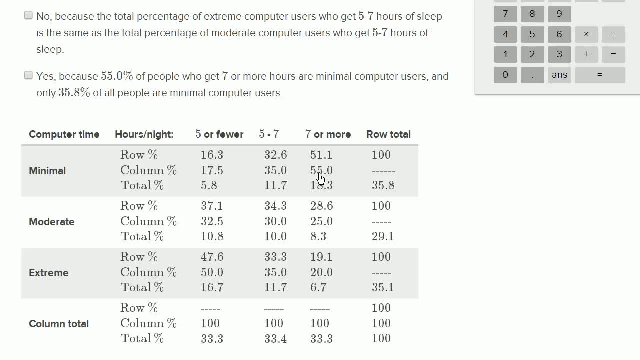 And there's three categories. So for 55% to be minimal computer users, it really does feel like the minimal computer users are more. they're definitely disproportionately representing the people who are getting seven or disproportionately represented in this category of seven or more hours of sleep. 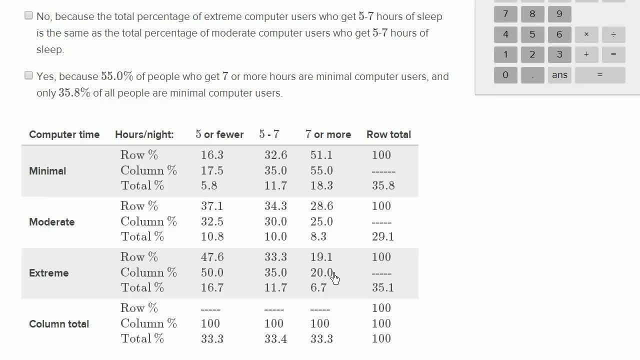 And you see that the extreme computer users in this category. they represent only 20% of this category, So it does look like there is an association between minimal computer use and getting seven or more hours of sleep. But let's look at the actual choices they give us. 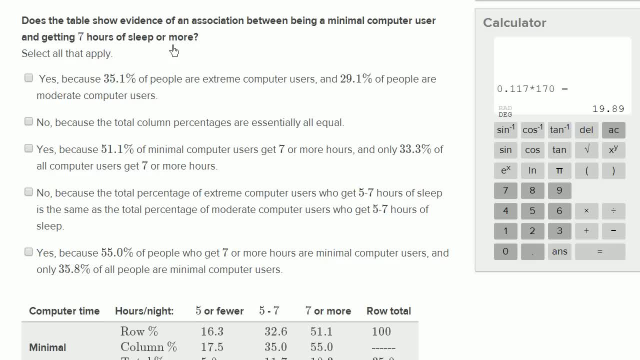 Does the table show Evidence of an association between a minimal computer user and getting seven hours of sleep or more? So yes, because 35.1% are extreme computer users and 29.1% of people are moderate. Well, I go with the yes, but this doesn't seem. 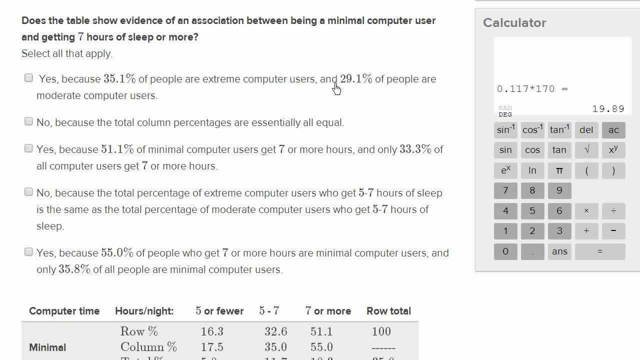 to really back up the claim. This is just giving us some kind of random data about the percentage that are extreme computer users or moderate computer users. No well, I explained why I go with yes, that there does seem to be a trend. 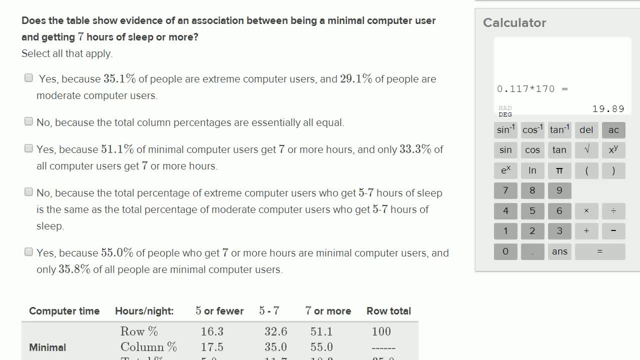 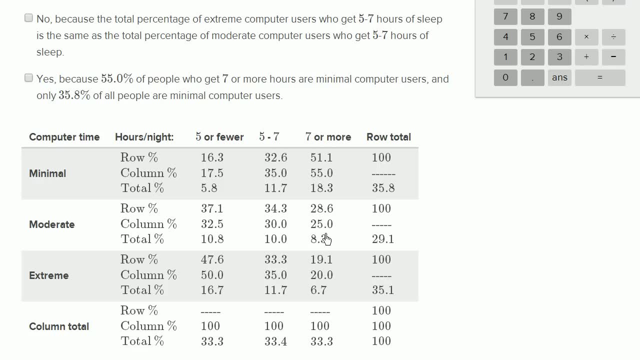 And I don't even believe what the statement is, because the total column percentages are essentially equal. We see that the column percentages are not equal for people who are getting seven hours or more of sleep, So we see that right over here: 55,, 25,, 20.. 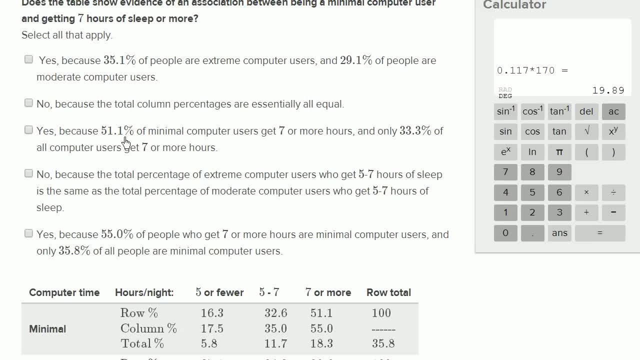 So I won't go with that one either. Yes, because 51% of minimal computer users get seven or more hours of sleep And only 33% of all computer users get seven or more hours. Yeah, I mean, that seems pretty good.